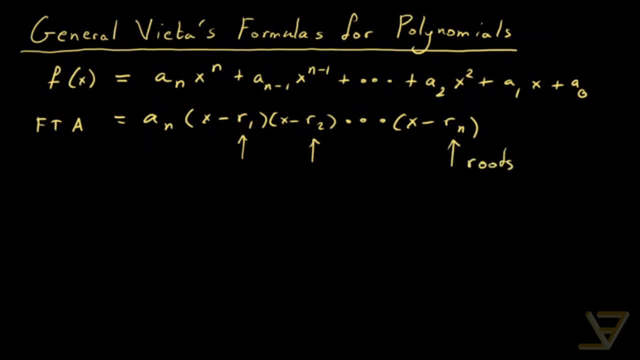 roots And some of them might repeat, in which case we say its multiplicity is greater than 1.. But when we write it out, the roots are r1, r2, all the way through to rn and we include the repeat. It's sort of like in a multi-set instead of a set, And what we want to do is relate. 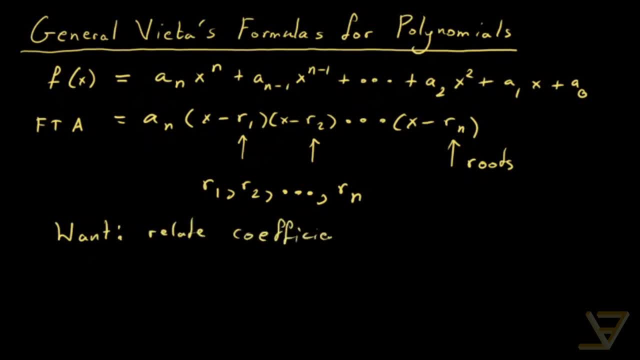 coefficients. These are an, an minus 1, all the way through to a2,, a1, and a0.. We want to relate them to the roots r1, r2, all the way through to a2,, a1, and a0. 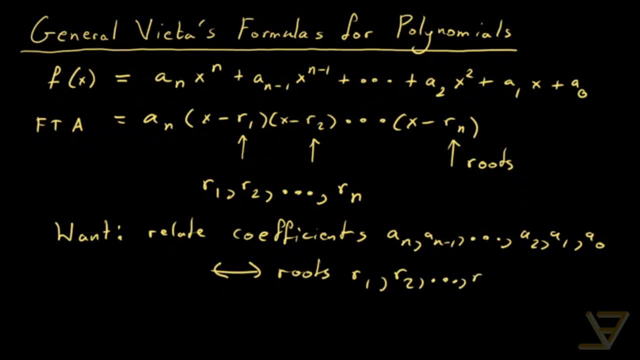 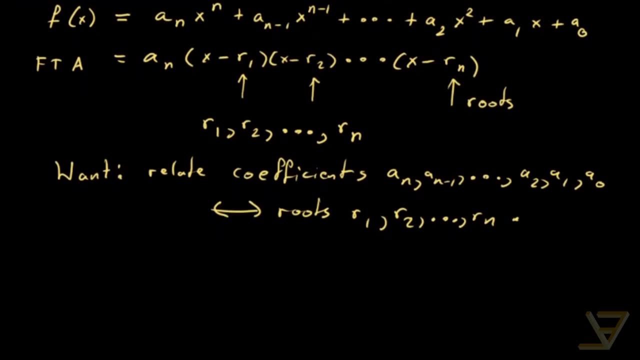 We want to relate them to the roots r1, r2 all the way through to a2, a1, and a0.. m out first minus rn, all the way through to a2, a3, and vice versa, And in a 2 ohm setting we separated them into two. weights i1, n. We want to create some equations that relate them together, And there is one general way of doing it, which is to take this equation and expand it, And then we're going to compare terms, coefficients, with this equation. so let's do an example. 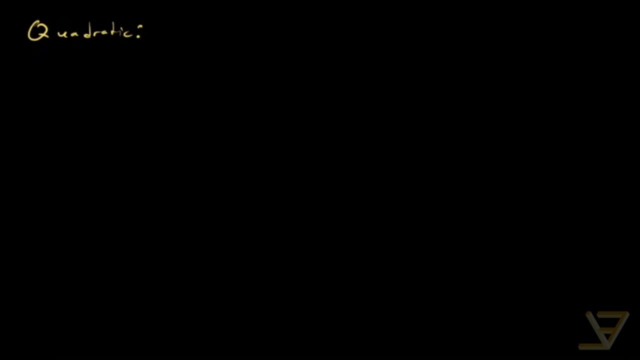 with a quadratic and a perfect out front x and aいうこと and an shortcut function tweet. Then we are going to out across the top of the 2 ohms square, which is a variable, and In the quadratic case what we have is that x squared, let's say we divide out by the leading coefficient, so that we get a monic. 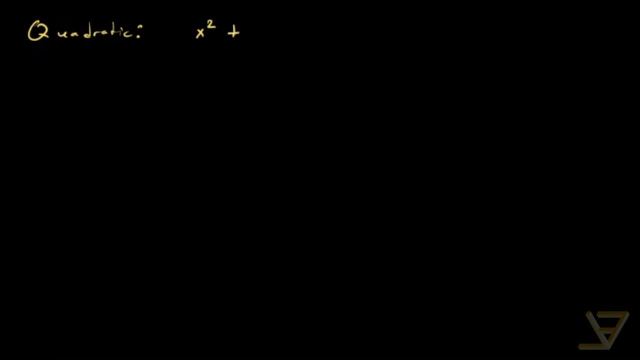 We get x squared plus a1 over a2, since we divide it out by the leading coefficient, x plus a0 over a2 is equal to, in factored form, x minus r1, x minus r2.. And notice that there's no coefficient of a2 over here, since we divide it out by it. 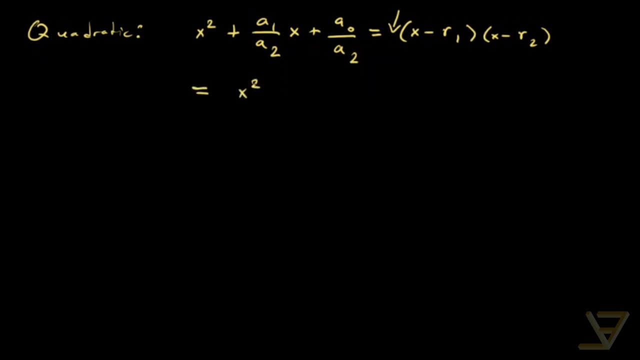 And if we expand it, we get that this is x squared Minus r1 plus r2, x plus r1, r2.. And now what we'll do is that we'll compare coefficients, So the stuff in the pink matches up. 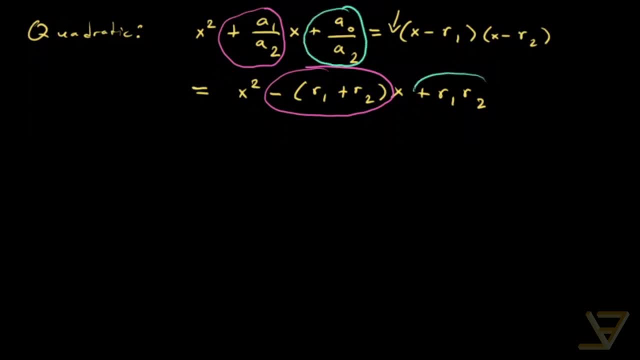 And then the stuff in the blue or light blue match up as well. So what we get is: r1 plus r2 is equal to negative a1 over a2.. And we also get that r1 times r2 is equal to a0 over a2.. 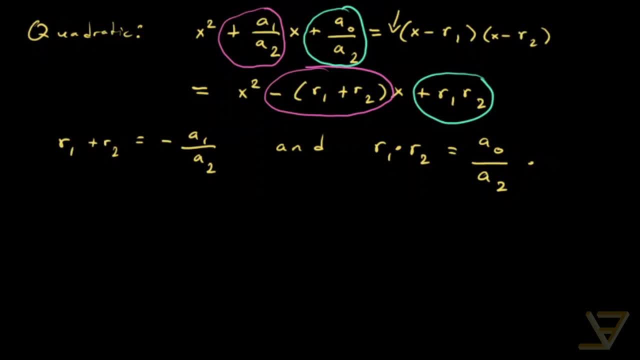 Let's repeat the exercise for a cubic before we move on to the most general case. So we have our quadratic up here. Let's do a cubic. Let's say we have x cubed plus a1 over. sorry, that's an a2 over a3.. 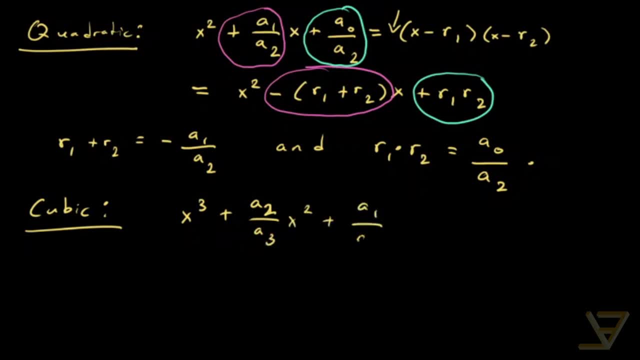 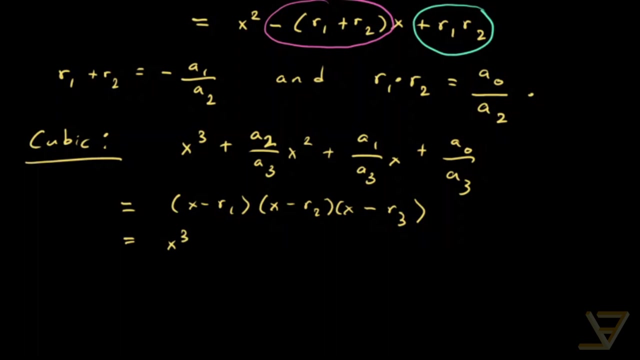 x squared. x squared plus a1 over a3x plus a0 over a3. And we're going to factor that as x minus r1, x minus r2, x minus r3. Now we're going to expand it, So we get x cubed minus r1 plus r2 plus r3.. 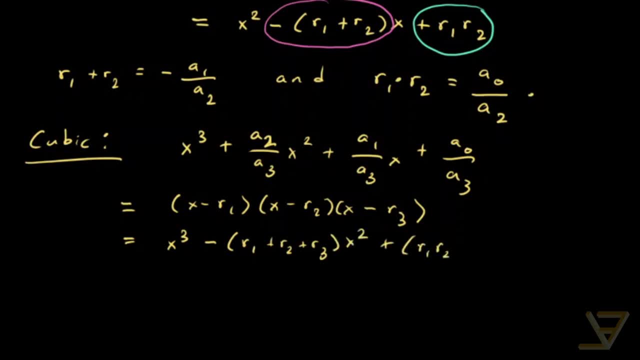 x squared, x squared Plus r1, r2, r1, r3, r2, r3, x, And our last term is negative: r1, r2, r3.. With the invisible x to the power of 0.. 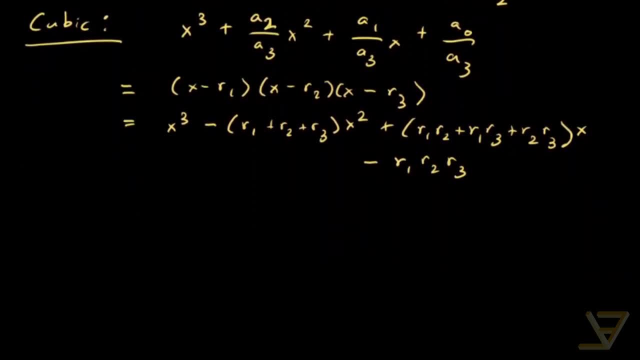 So let's compare coefficients. We have a2 over a3.. And negative r1, r2, r3 as a sum. So r1 plus r2 plus r3 is equal to negative a2 over a3.. Then we have a1 over a3. 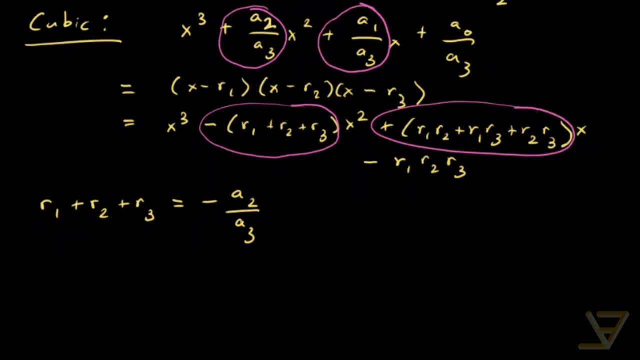 And this symmetric sum over here, So r1, r2 plus r1.. R3 plus r2, r3 is equal to a1 over a3. And the last one is a0 over a3. And we match that to negative r1, r2, r3.. 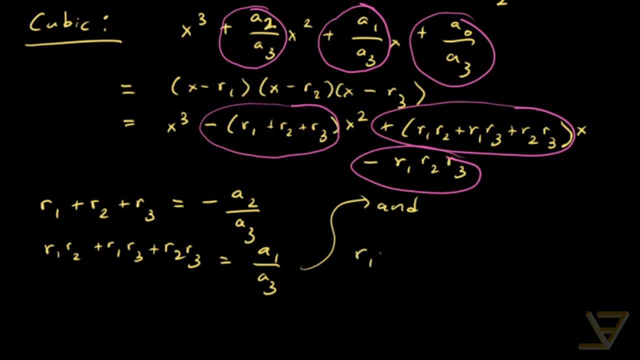 So we get r1, r2, r3 is equal to negative a0 over a3.. So just a couple of patterns here. First of all, we have alternating terms, So we have negative here, a positive here and a negative here. 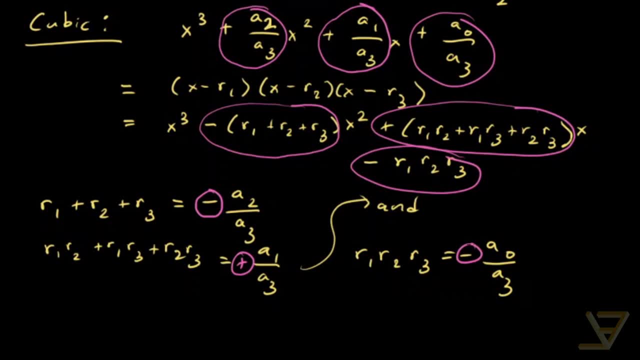 So it looks like we're going to have negative 1 to the power of k of some sort, And the other thing is that these sums that we have, they're symmetric in the roots involved And that's why we call them symmetric sums. 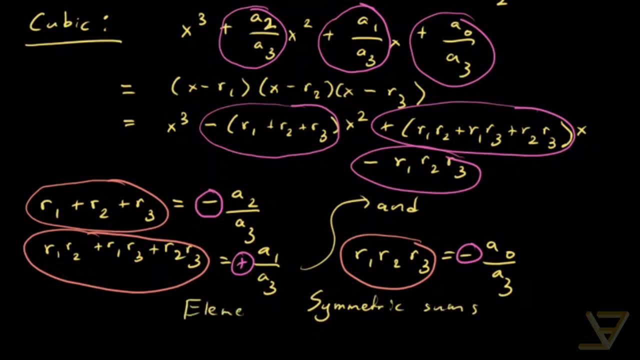 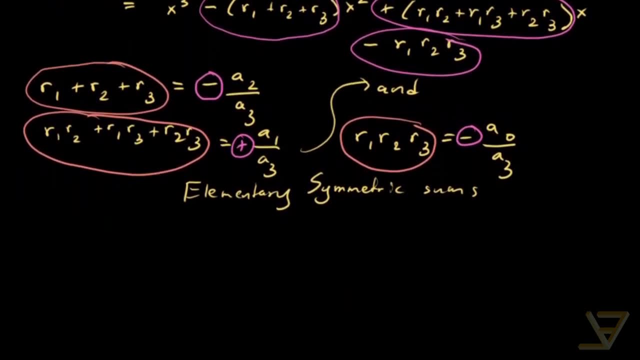 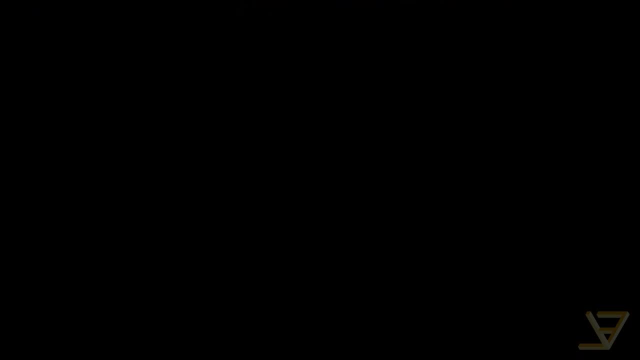 In fact we call them elementary symmetric sums, Because out of these symmetric sums we can build all other symmetric sums. I believe that's called the fundamental theorem of symmetric sums. Okay, so we focused on a few small cases. two small cases. 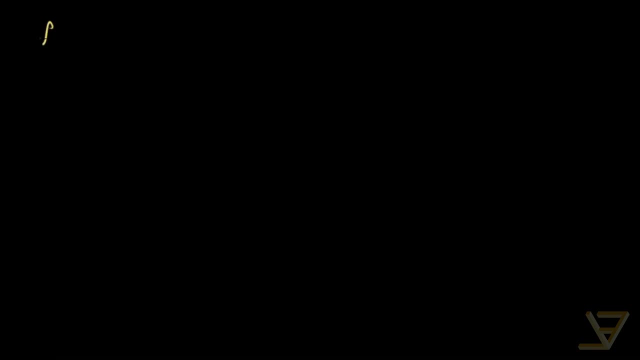 And now we're going to look at the general idea. So the general idea is that if f of x equals to a1, a n, x to the n plus a n minus 1, x to the n minus 1, all the way through to a2, x squared plus a1, x plus a naught. 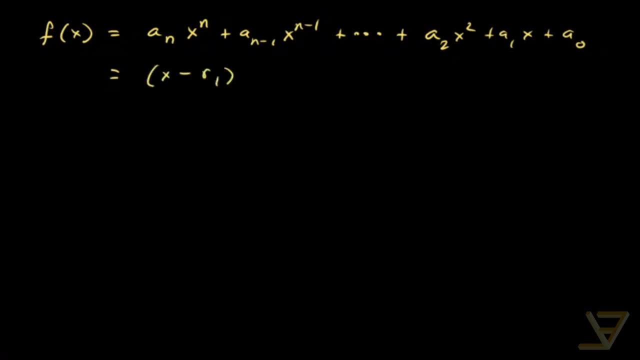 and that is equal to x minus r1, x minus r2, all the way through to x minus rn, with a coefficient of a n out here We're going to divide out by a n, So we get x to the n. is x to the n plus a n minus 1 over a n x to the n minus 1,. 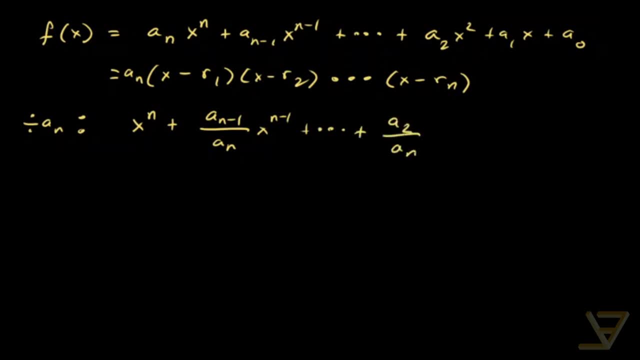 all the way through to a2 over a n, x squared plus a1 over a n, x plus a naught over a n, And that's going to equal x minus r1, x minus r2, all the way through to x minus. 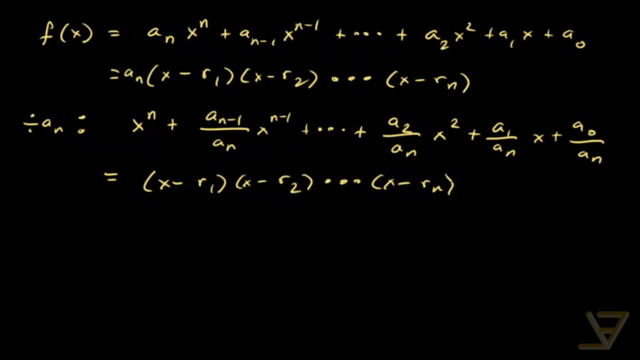 plus a1 over a n, And now we're going to expand it. So let's look at the coefficient of x to the n minus k, for k equals to 1,, 2,, 3,, all the way through to n. 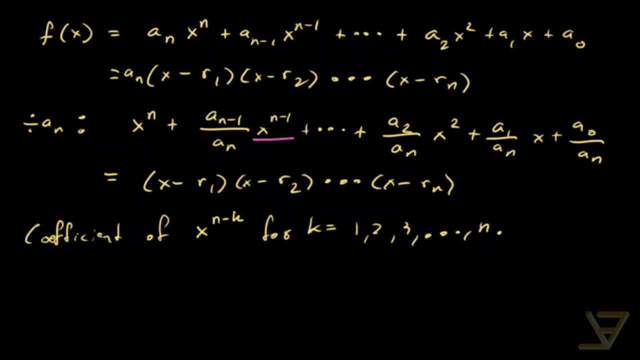 So we're going to be looking at the coefficient of this all the way through to this, this and this. And now. the rules of expansion say that if we have x to the k- sorry, n minus k- then the other k terms will choose some of these negative ri's. 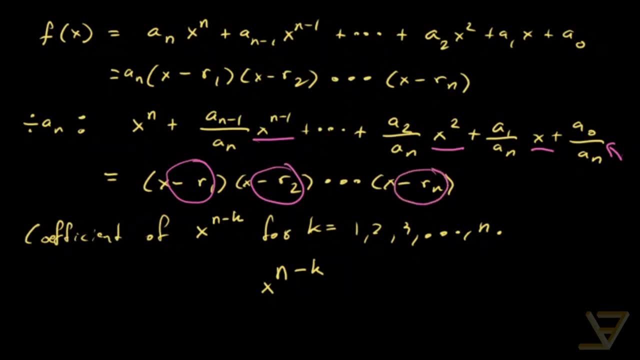 So we're going to have k of those that we're going to choose. So what that is going to equal is the following coefficient: It's going to be the sum over the k tuples. so i1 less than i2, all the way through to ik. 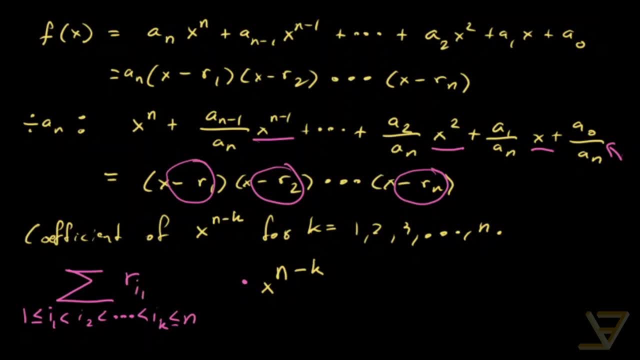 less than or equal to n, And we're going to have ri1,, ri2, all the way through to rik, and that's going to be the coefficient of this And And that in turn. I'm sorry there's also a negative 1 to the power of k. 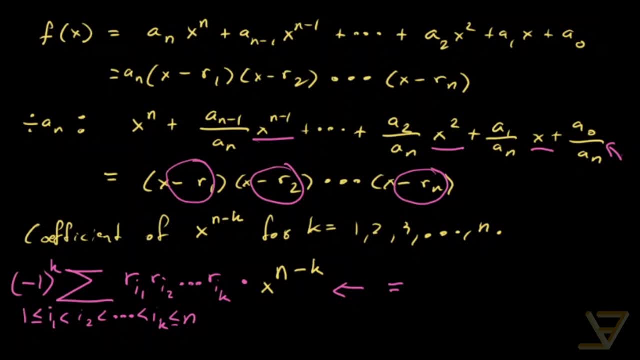 That's actually really quite important. that accounts for these negative signs and the alternating pattern that we saw earlier And that's going to equal a n minus k over a n x to the n minus k. So really we can get rid of these x to the n minus k. 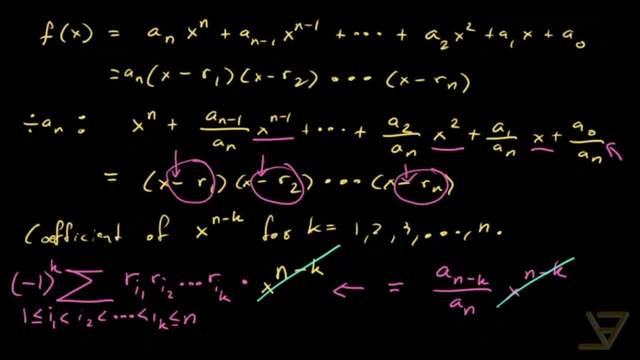 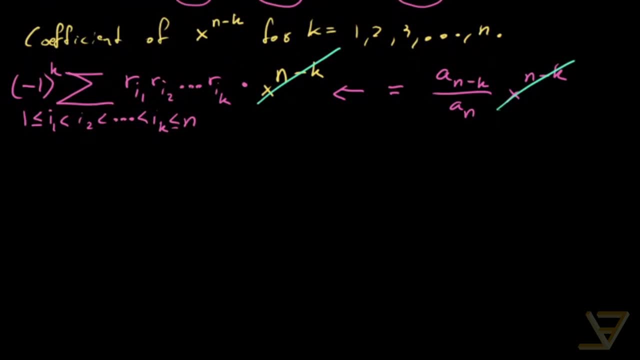 Just know that that's the coefficient, that's the term whose coefficient we're looking at. So that is Vieta's formulas, that you have an equality between this almost disgusting looking sum versus the ratio of these two coefficients. And I just want to show you an easier way of writing this. 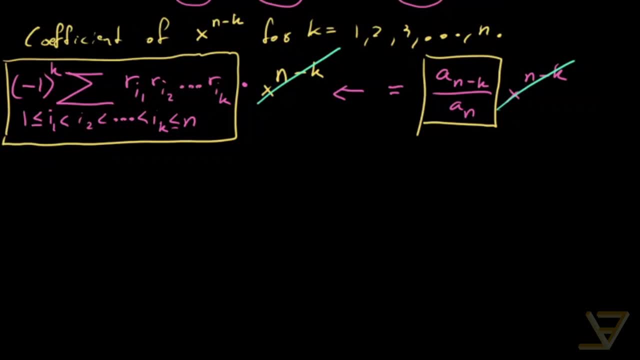 It's a bit more of an advanced way, but it is easier. You avoid a lot of the indices. So we have this sum here: negative 1 to the k times 1 is less than or equal to i1, less than i2, less than all the way through to ik, less than or equal to n. 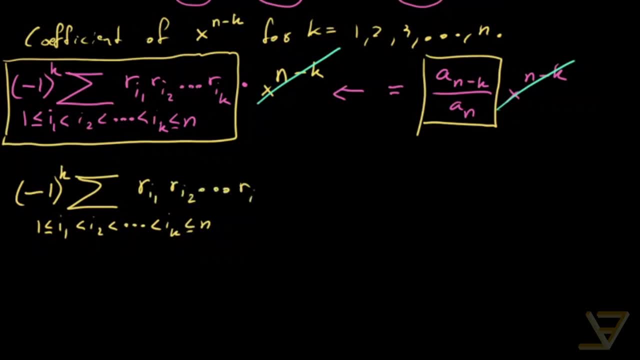 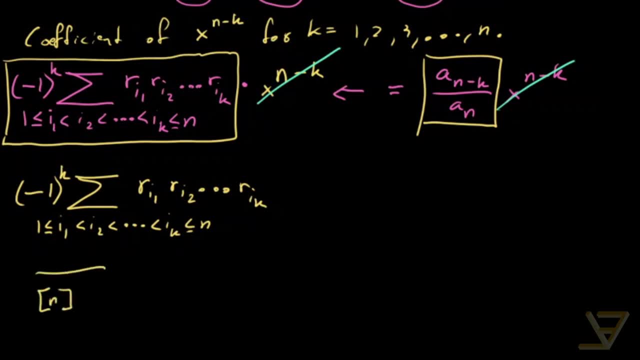 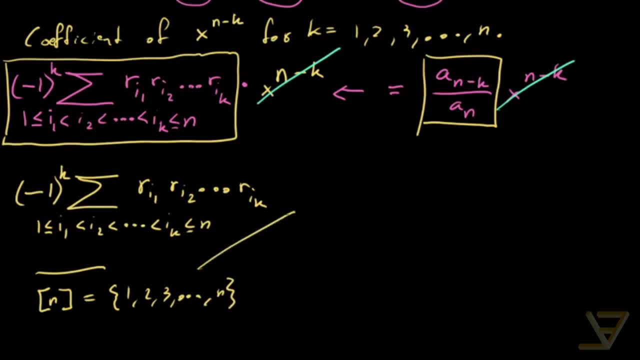 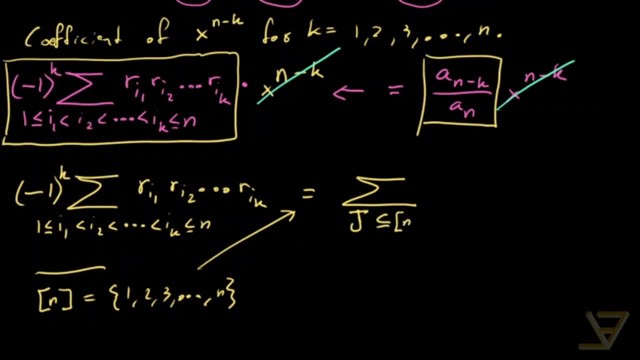 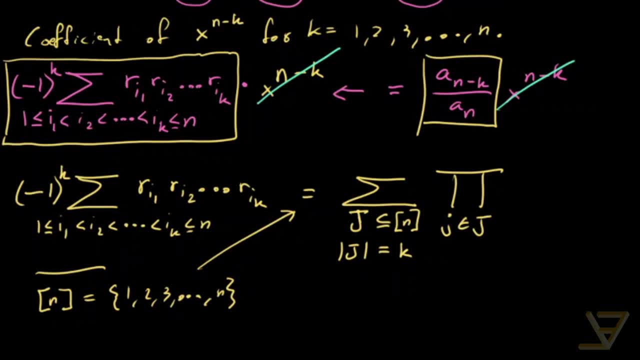 take the product of the elements of J, and those are the ij's, and of course we have a coefficient of negative 1 to the K, and that will equal a n minus K over a n. so I just want to show you this, the second way of writing this sum of: 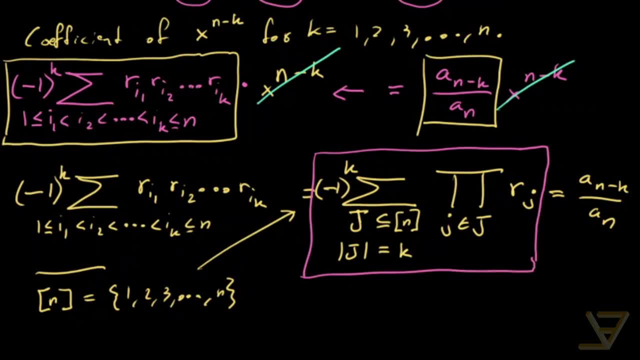 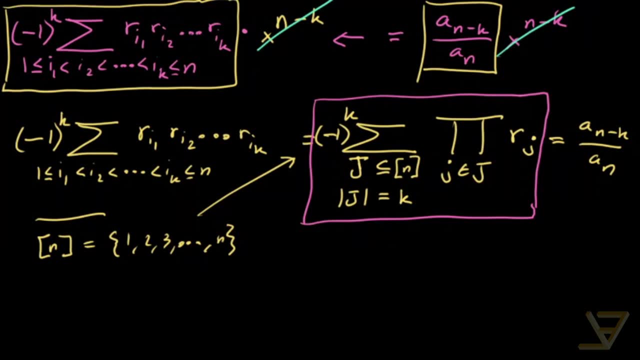 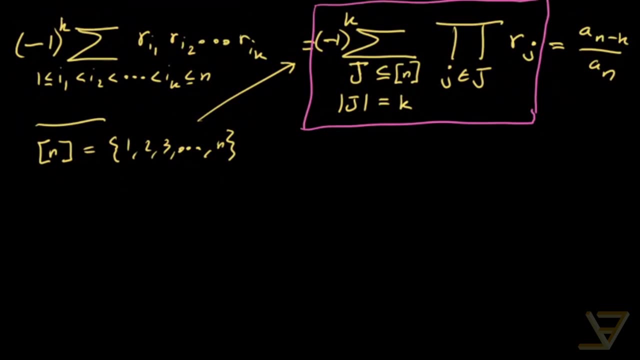 products, because this, this kind of way of writing things, does come in handy, for example in the principle of inclusion exclusion. so before we end, I'll show you a couple of concrete examples, which are the two most important examples. the first one is for the sum of the roots. so we get r1 plus r2 plus r3 is all the way through to rn. 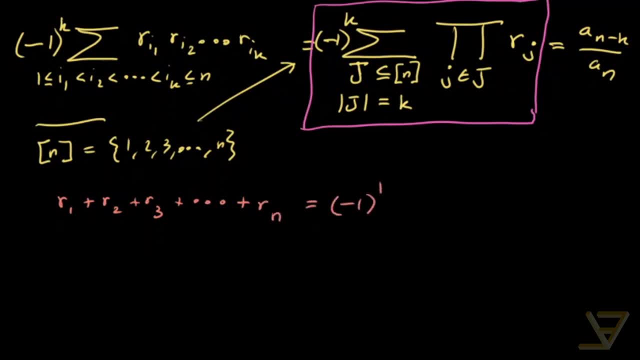 is equal to negative 1 to the 1 of a n minus 1 over a n. notice that this negative 1 to the K, I brought it over here. that's actually the traditional way of writing it- and this is equal to negative a n minus 1 over a n and the.